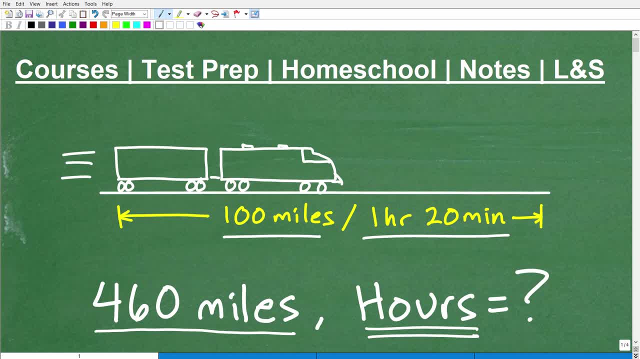 that all students can be successful in mathematics, But it requires math instruction. You've got to be learning from a teacher that you really understand. So that's clear, understandable and comprehensive math instruction. That's what you need to be successful in mathematics. So if you need help in your current math course or some sort of special, 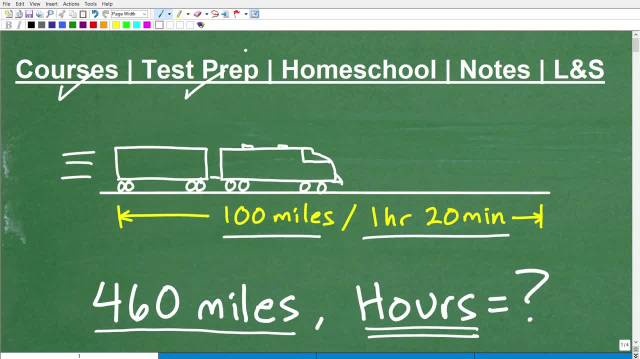 test that you're studying for, maybe something like the GD, SAT, ACT, ASVAB, teacher certification exam, anything with math on it. or if you're homeschooling math, check out my math help program. I'm going to leave a link to it in the description of this video. I promise it will help. 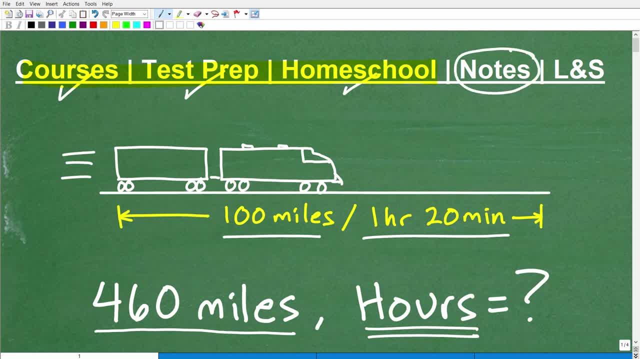 you out big time. Also, I'm going to leave links to my math notes in the description of this video, But you should be taking your own awesome math notes. Note taking is so important when you're learning anything, not just math, any academic. 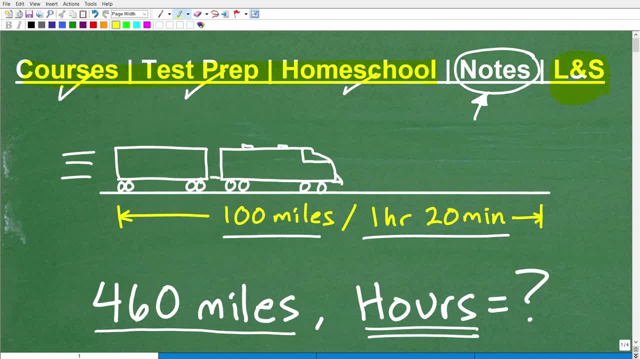 subject: You want to be a great note taker, And if this video helps you out, don't forget to like and subscribe, as that definitely helps me out. OK, so I'm going to go in and show you the solution to the problem right now. 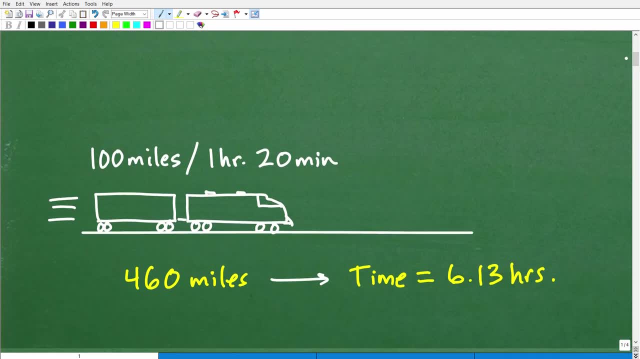 And then we're going to get into exactly how to solve this. All right, So here's our train, the train. It took one hour and 20 minutes to go 100 miles, So 460 miles. How long will take that train in terms of hours? 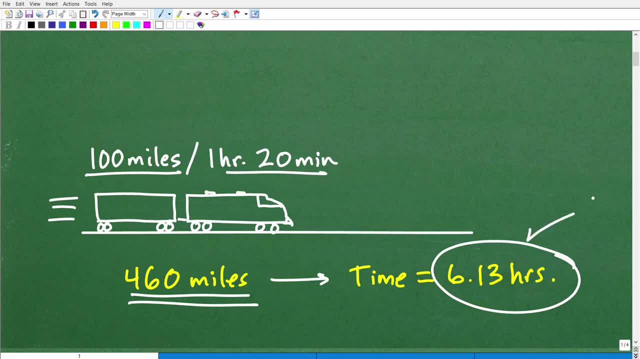 Well, 6.13 hours, that is the correct answer. So of course this is kind of rounding off a bit of a decimal, But it should be your answer. your correct answer should be somewhere pretty much approximately equal to 6.13.. 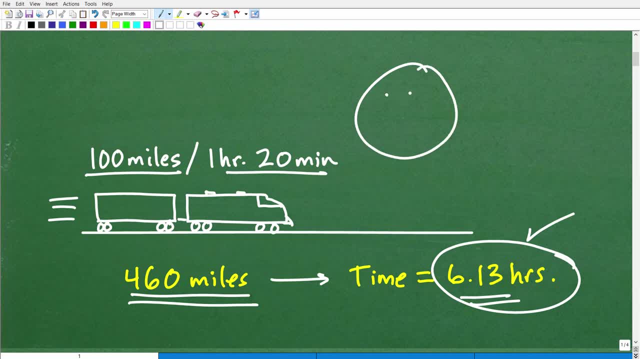 OK. So how'd you do? Well, if you got this problem right, Let me go ahead and give you a nice little happy face and a plus, plus, because this is a word problem- a 100 and multiple stars for being so awesome at basic algebra- word problems, so nice job. but if you are confused, we'll stick. 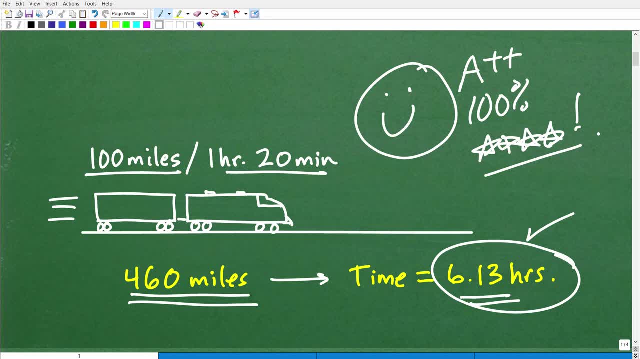 around for a couple minutes. you're going to learn exactly what to do now to solve this problem. we're going to need a formula, okay, so that's one thing we're going to need to know, and kind of the um, the main idea to solve this problem is finding the speed of the train, okay, so here we know how. 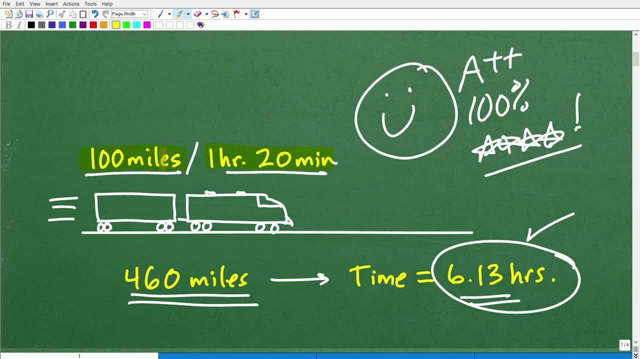 long it took this train to go a particular distance. all right, but we don't know the speed of the train, so that's going to be a key component here. how do we find the speed or the rate of this train? well, i'm going to get into a second, but once we get into that, in a second. but if we know the, 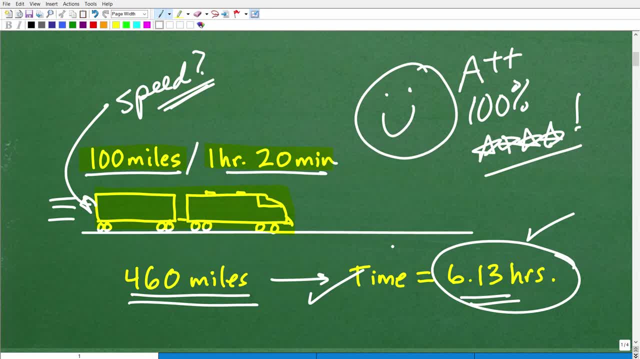 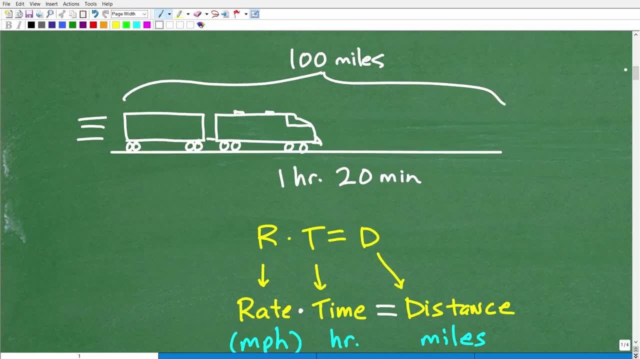 speed of the train, then we can easily calculate this part of the problem. okay, so let's go ahead and get into this now. all right, so what do we know? what are the facts? well, we know that this train took one hour and 20 minutes to cover 100 miles. okay, great, but again. 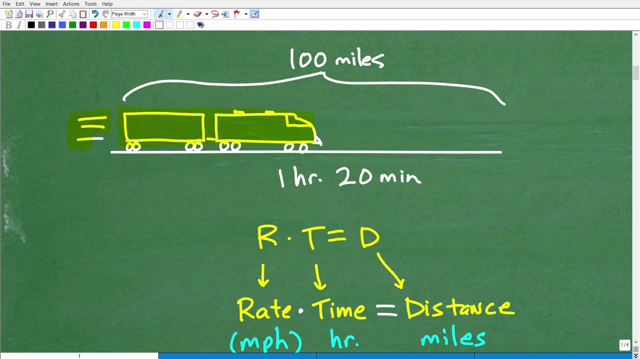 i want to know the speed of the train. okay, what is the rate or the speed? well, you want to be familiar with this formula. all of you out there that are studying algebra need to know this formula right here. okay, rate times- time is equal to the speed of the train. okay, so let's go ahead. 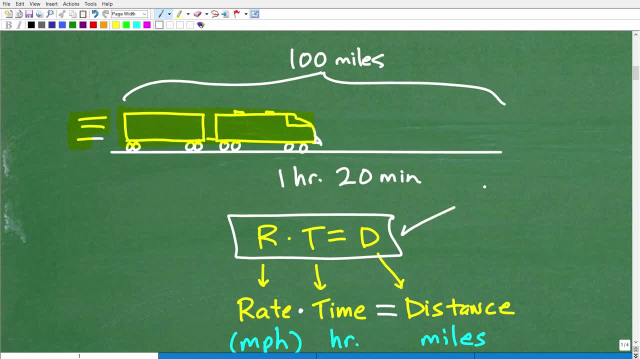 and look at this formula. okay, school to distance: put this in your long-term memory. ie um know this formula so well where you don't have to like look at a formula sheet to remember it. okay, there's some formulas in mathematics that you just want to commit to your long-term memories. this is one of 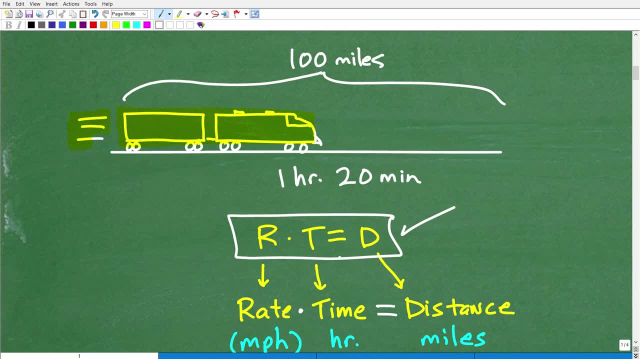 them. okay, there's so many motion or speed, rate and time problems. this is the formula that you need to know to solve all those problems. but let's go ahead and talk about how to use this formula, and then, of course, we'll go to the next slide and we'll talk about how to use this formula, and then 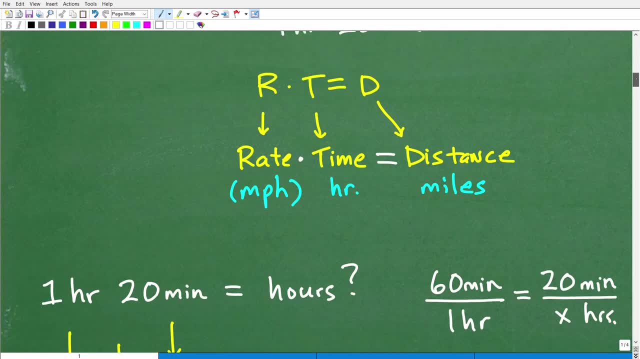 circle back and actually apply it here. okay, so rate times. time equals distance, so let's talk about rate. rate is effectively your speed, okay, velocity. so if you're told like the velocity of something or the speed of something, or the rate of something or how fast something's going, that 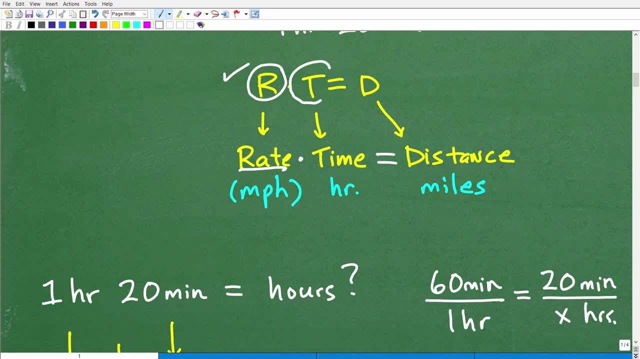 is your rate. okay, now time is, of course, time, all right. and then d is distance, but here's the key. okay, we have to be very, very uh uh concerned with our units of measure when we're using this formula. all right, so let's talk about distance. so here we're talking about miles, in this particular 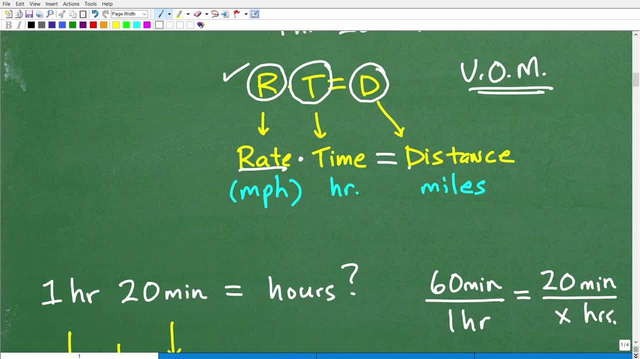 problem. right, the train went 100 miles, or how long did it take? the train go 460 miles. so our unit of measure here for this particular problem is miles, okay, not feet, not inches, it's miles. we're also talking about hours, okay, so when we're looking at our rate, 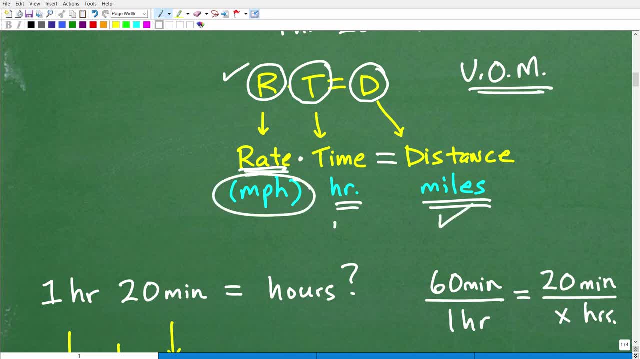 respective rate. we're going to be thinking about miles per hour, okay, miles per hour. so you're like: okay, hours and miles, miles per hour. now, miles per hour, this is what we call a rate in mathematics and effectively this is miles, uh, per one hour. okay, how many miles do we go per one hour? per 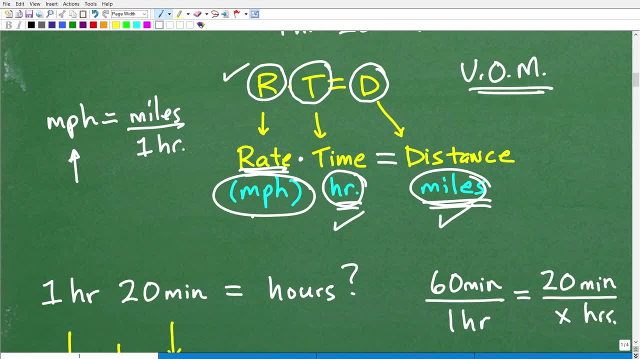 one hour, that's miles per hour. of course, we more commonly write it this way. now i could solve this problem by using this formula here: okay, so we're going to be thinking about miles per hour for r here. okay, let's actually do that now. let's use some basic algebra, so here we have rate times. 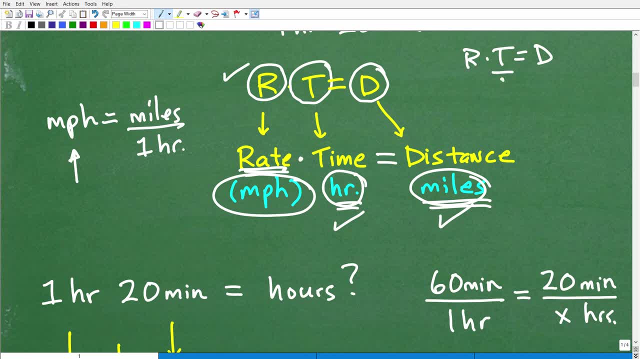 time is equal to distance. if i solve for rate, i'm going to divide both sides of the equation by t, okay, so, uh, just right, we can effectively rewrite this equation as r is equal to d divided by t. okay, so why did i do that? well, i want to really kind of emphasize units of measure here. so my rate. 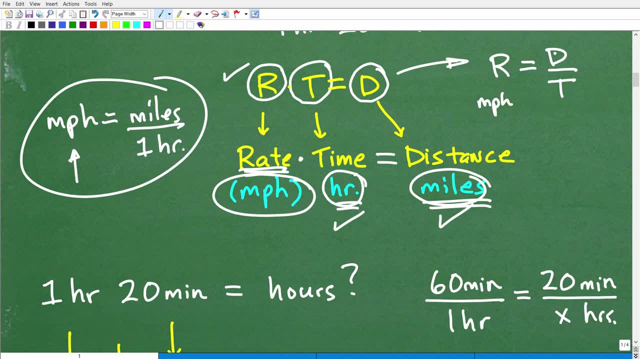 is in the middle of the equation and i'm going to divide both sides of the equation by t and i'm going to divide both sides of the equation by t and i'm going to divide both sides of the equation by t per hour. and we could better see that here with this equation, because my distance would be in. 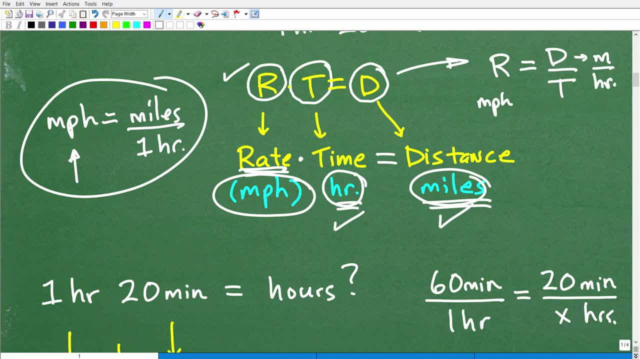 miles and my time would be in hours, so that's miles per hour. so again, very, very important that you understand units of measure, because this is typically, uh, where students kind of would, um you know, go wrong or make errors with this particular formula. they might know the formula, but they're. 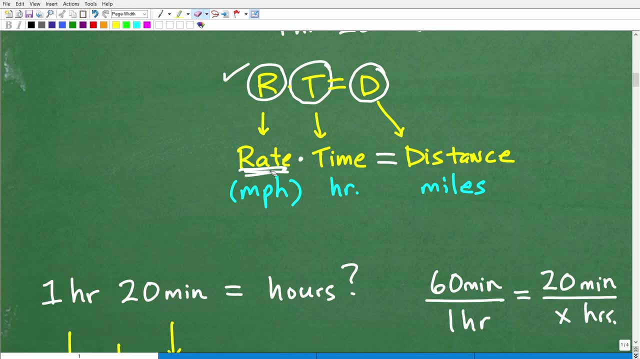 not using the correct units of measure. so again, that's why i'm really, really spending a lot of time to do this. so i'm going to divide both sides of the equation by t, and i'm going to divide both sides of the equation by t, and i'm going to divide both sides of the equation by t and i'm going to. 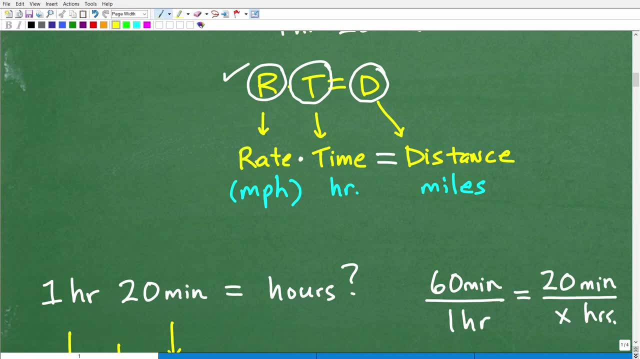 this point home, okay, so let's go ahead and talk about this now. so my time has to be in all hours, okay, my distance has to be in all minutes, and so when i use this formula, i will be able to figure out the speed of the train in terms of miles per hour. but here's the deal. okay, i need all hours. 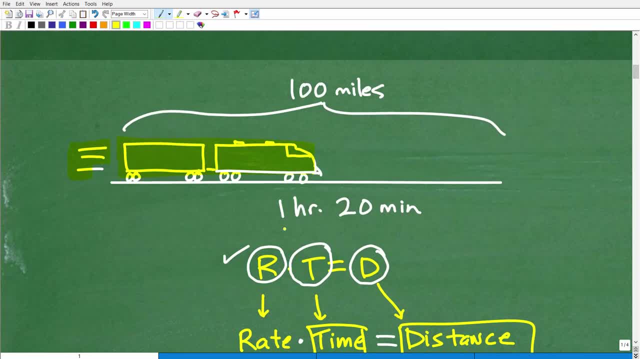 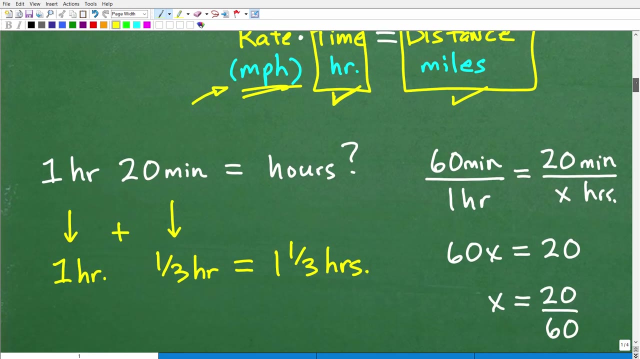 but i do. i have all hours here. no, i have one hour and 20 minutes. so i'm going to have to fix this up, because time measurement is in all hours. okay, all hours, not hours and minutes. so that's our first task here, okay, so let's go ahead and get into this. so, one hour and 20 minutes, how many hours is this? 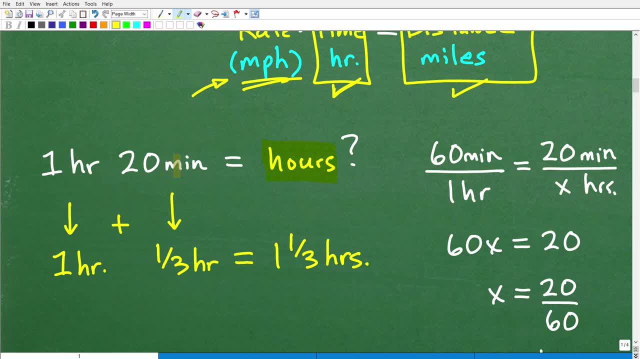 not how many hours and minutes. yeah, we have an hour here and 20 minutes here, so we're gonna have to figure out how much of an hour is. 20 minutes? okay now, hopefully some of you can be like: well, 20 minutes is just one third of an hour, because 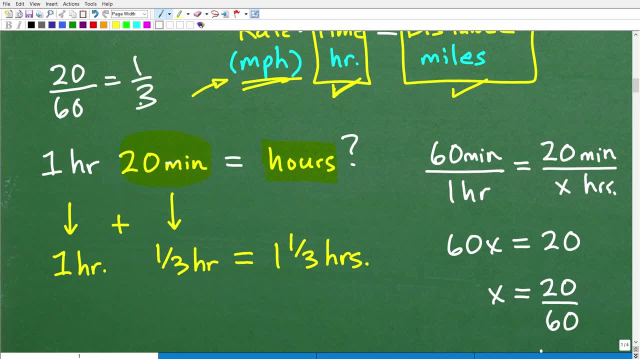 out of 60. So if you were able to kind of reason that 20 minutes is one third of an hour, that's excellent. But if you need more of a technical way to do this, you could set up a nice proportion. So let's go ahead and take a look at this right here. So 60 minutes is to one hour. Okay, there's. 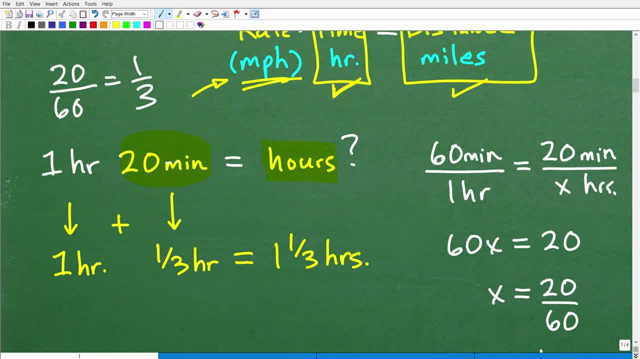 one hour in 60 minutes, And what I'm doing here is a proportion, Okay, and that's the same as 20 minutes is to how many hours Okay. So if you're not sure how to do this part of the problem, you. 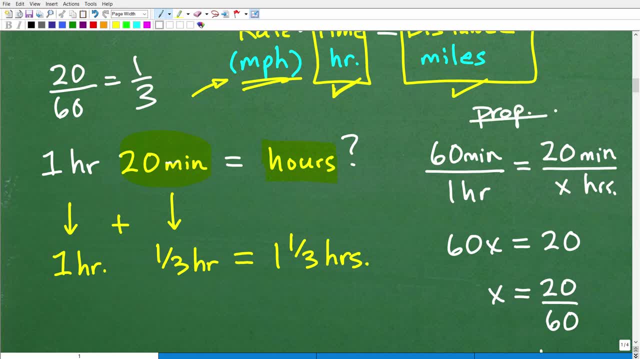 want to go ahead and review proportions. Okay, so we can set up a proportion Again: 60 minutes is to one hour, as 20 minutes is to how many hours. So what we can do now is simply use the cross product to solve this proportion. So x times 60 is 60x. one times 20 is 20.. And I can solve for x. 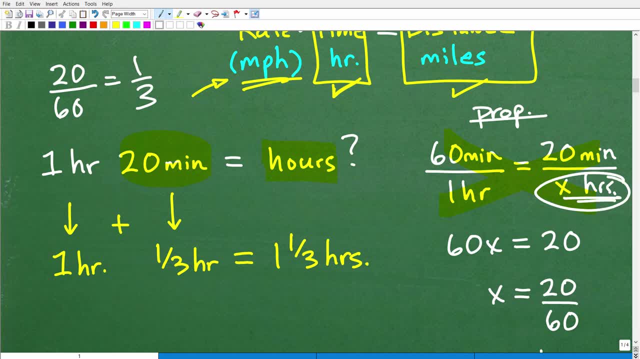 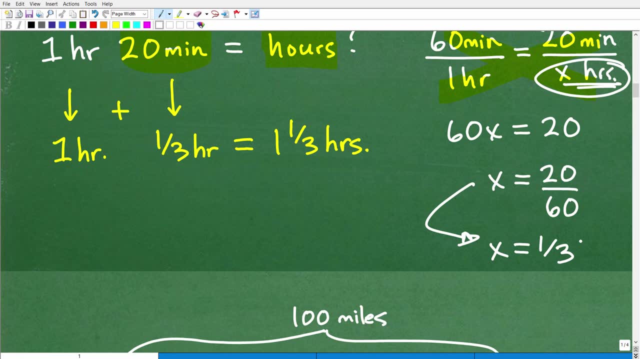 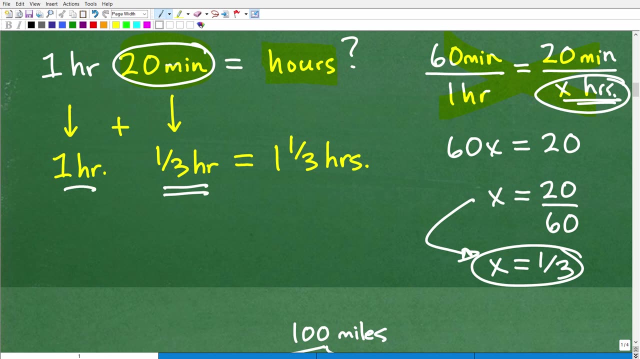 and x is going to be its units of measure. it's going to be our hour, So I get: x is equal to 20 over 60, which, of course, I can reduce to the fraction one third. Okay, so I now know that 20 minutes is one third of an hour. So one hour and 20 minutes is one plus one third. 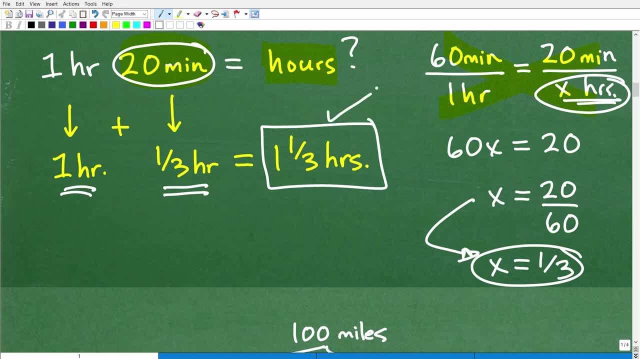 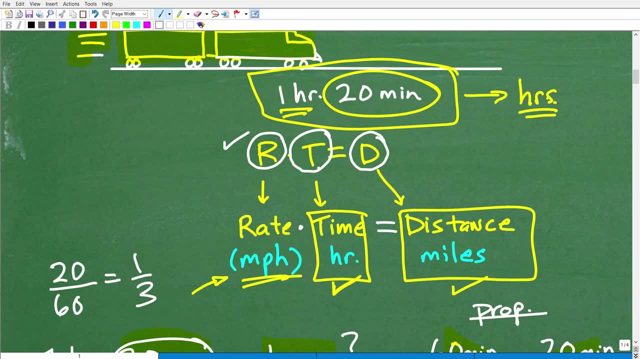 or one and one third hours. Okay, All right. So that's really our first move to figure this thing out, Because I'm looking at this formula. my first thing is: okay, great, I want to use the formula, But I got a first. 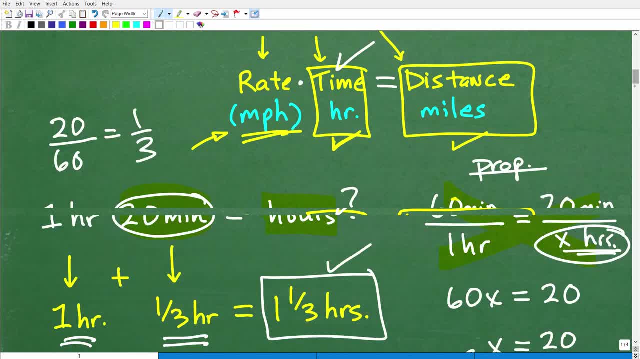 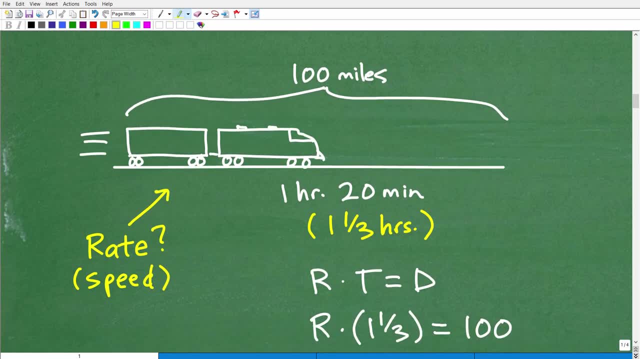 so let's look at the formula. So let's say one hour and 20 minutes, Okay, and let's go ahead and take a look at the problem this way, Right? so here's our train. It went 100 miles, And how long. 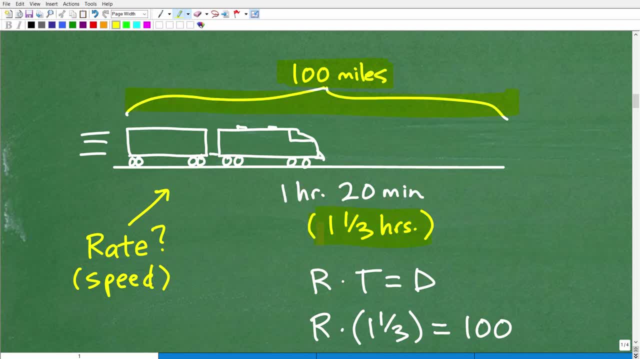 well now. it went in one and one third hours. we know it's an hour and 20 minutes, But now we have all miles and all hours, So I can figure out the rate or the speed of this train in terms of miles per hour. So let's go ahead and do that now. 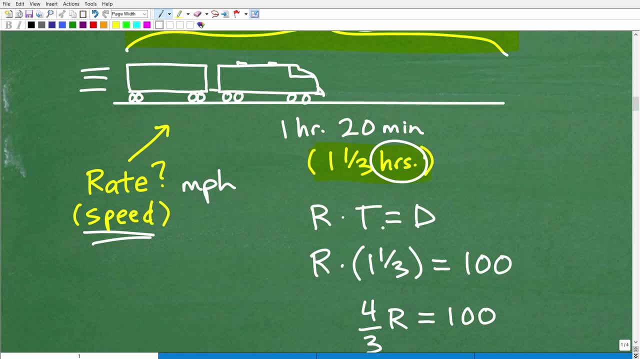 Now, so let's use the formula Rate times. time is equal to distance, So what is the time, Okay? well, the time is one and one-third hours. Okay, so I'm going to replace that t with the one and one-third. 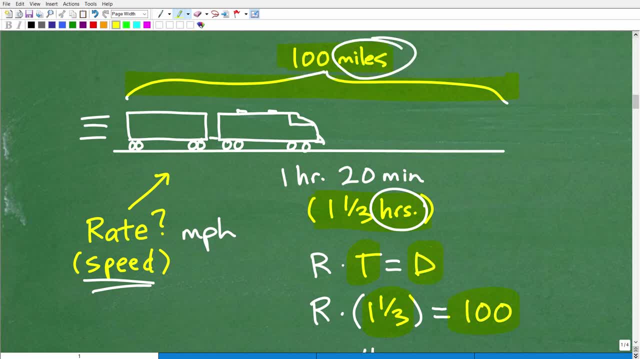 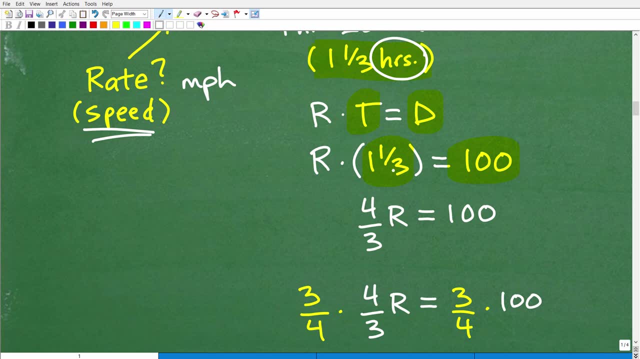 And what is the distance? It's 100 miles, right, 100 miles. So I'm going to go ahead and solve for r right Now. the easiest way to do this algebraically is to change this mixed number fraction into an improper fraction. 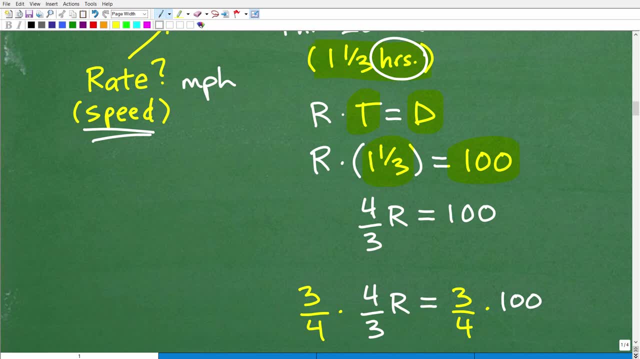 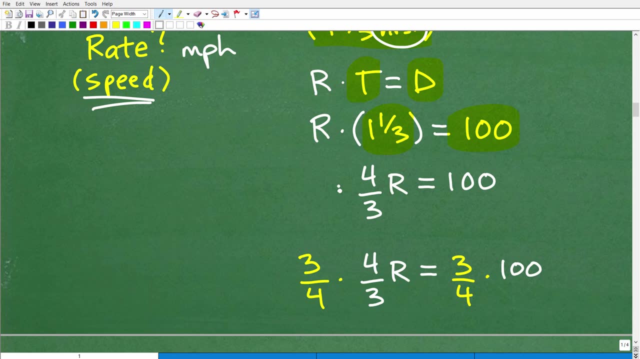 So three times one is three plus one is four. So this is the same thing as four-third times r is equal to 100.. So to solve this basic algebra equation the easiest thing to do is to multiply both sides of the equation by the reciprocal. 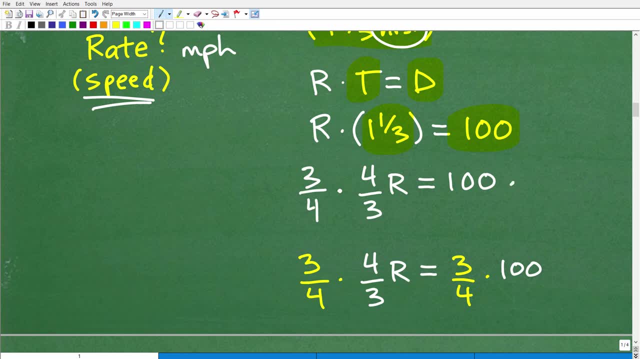 Okay, you could divide both sides of the equation by four-thirds. It's the same thing as multiplying both sides of the equation by the reciprocal. So again, if you're confused about this part, right here what I'm doing, you need to solve or you need to review the basic equation. 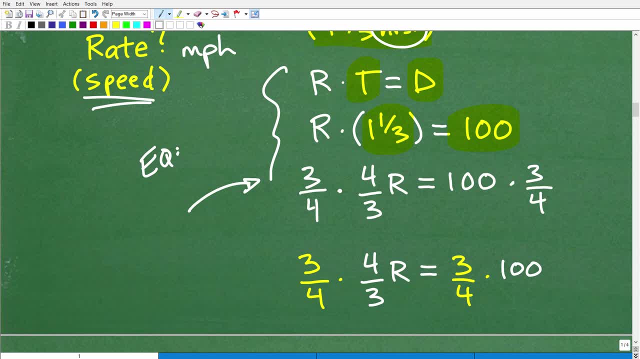 So remember this is an algebra word problem. We're applying math skills that you should already know, So if you're lost, you probably need to review basic equations, proportions, etc. All right so, but if you understand this, we can solve for r. 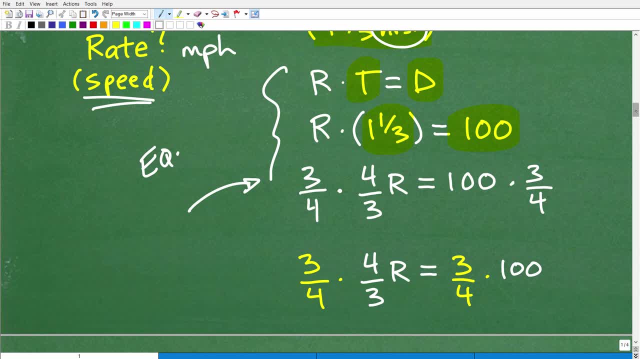 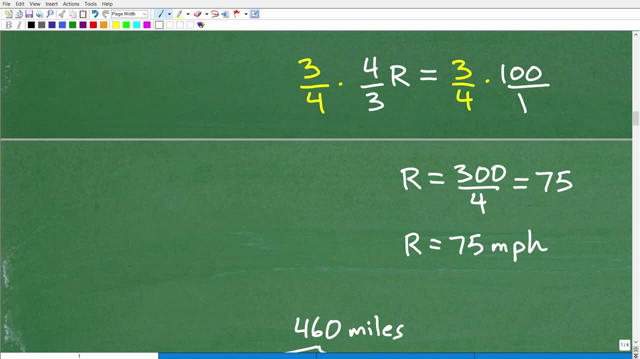 Just simply multiply both sides of the equation by three-fourths And let's take a look at the answer. All right, so r is going to be equal to. this is a fraction right here: 300 over four. 300 divided by four is 75.. 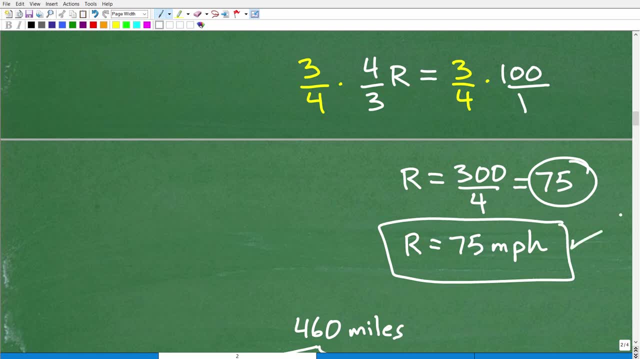 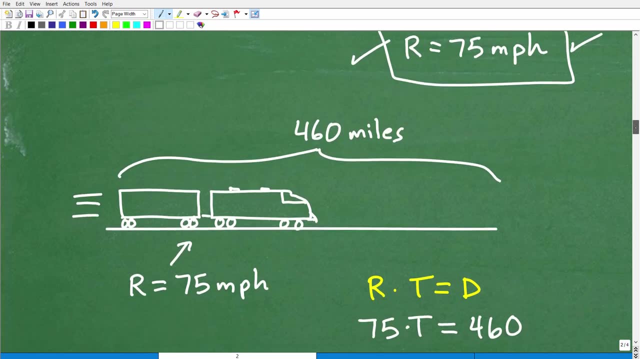 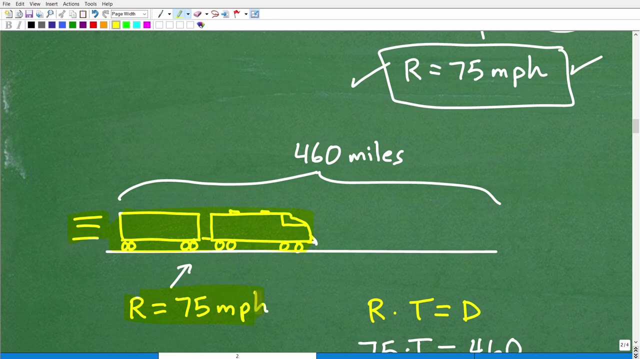 But again we're thinking about units of measure. So the rate is 75 miles per hour. Okay, that's how fast our train is going. Okay, so now that we know how quick or how fast this train is going, the rate of the train: this train is going 75 miles per hour. 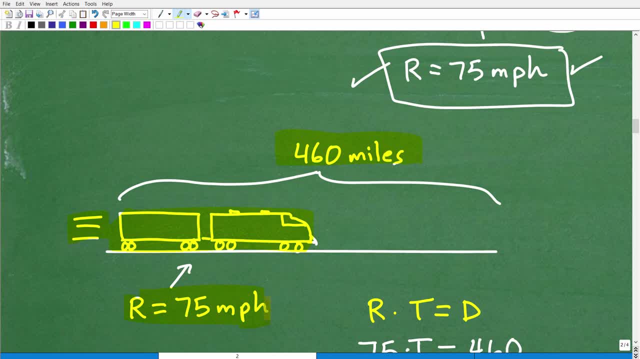 Okay, how long will a train going 75 miles an hour take to cover 460 miles? Well, this here It's going to be nice and easy, because this units of measure is in miles, And here we have miles per hour. So when we use the rate times time equals distance formula, our answer is going to be in hours. 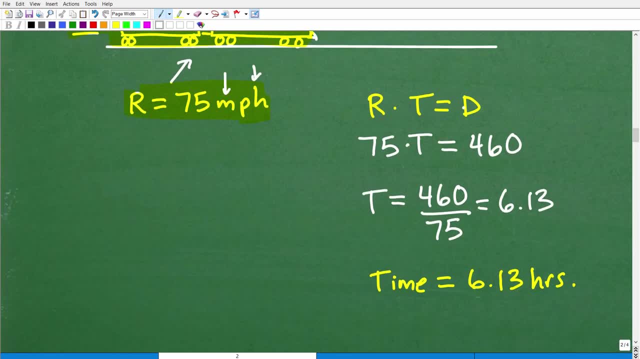 And that's what we want. So let's go and figure this out. So rate times: time is equal to distance. We know the rate. Okay, the rate is 75 or 75 miles per hour. T is what we're looking for, right. 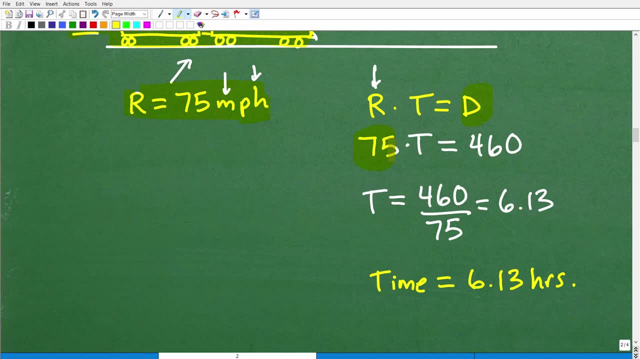 And this is going to be in hours, because this is miles per hour And our distance is in miles, And so this is already set up nice and easily for us, or nice and correct, because we already did the work up front. So to solve for T, I'm going to go ahead and divide both sides of the equation by 75.. 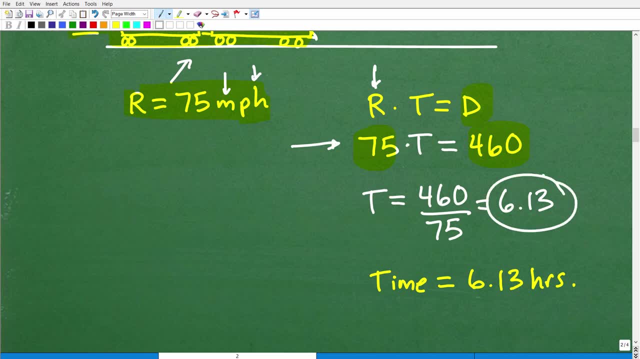 So that's going to be 460 divided by 75,, which is 6.13.. And again you need to understand what is the unit of measure. that's in hours, And that's what we're looking for. So there you go. 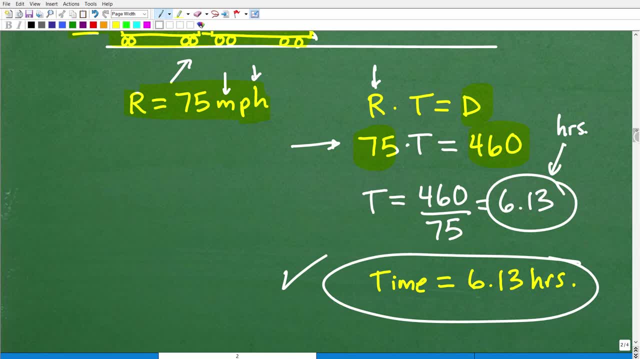 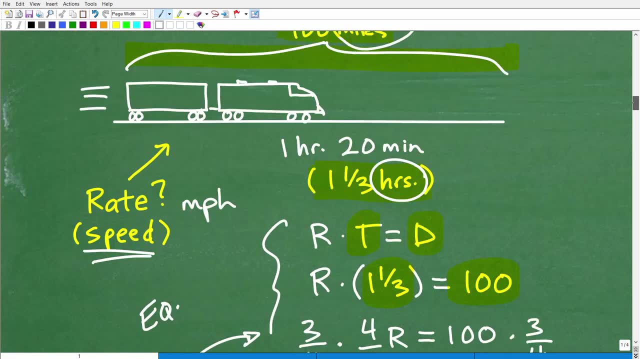 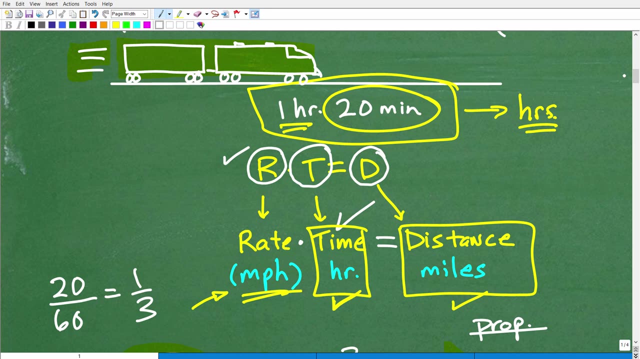 Okay, All right. So probably this problem, Okay, I would say for a lot of you, probably the point that you need to work on. Well, it's actually going to be a couple of things. So the first thing I would strongly suggest you make sure you understand is working with units of measure. 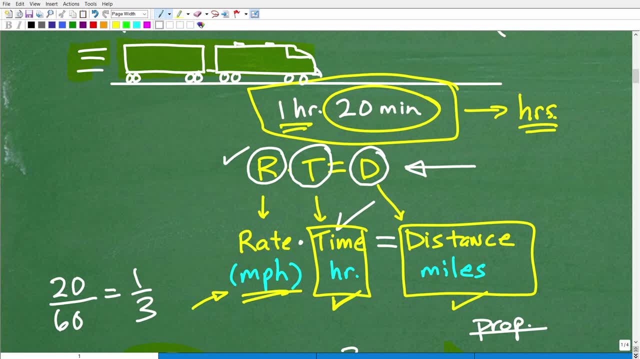 When you're working with particular formulas, any formula, physics, math doesn't make a difference. You want to be thinking about units of measure and how to convert one unit to another. Right, And of course, I can't explain all these things in this one video. 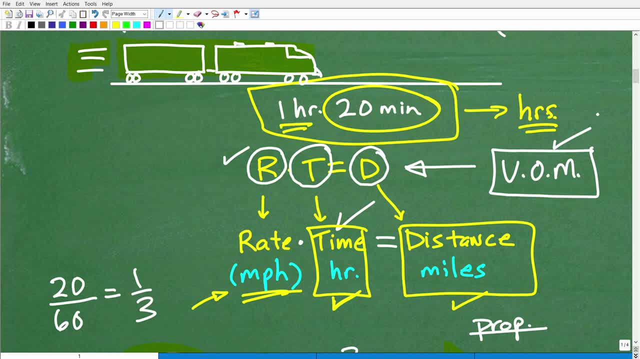 I'm just kind of highlighting different skills that you need to be aware of. So that's the first one. The second thing is you need to know how to solve equations- Okay, Various equations- and solve for specified variables in a particular formula as well. 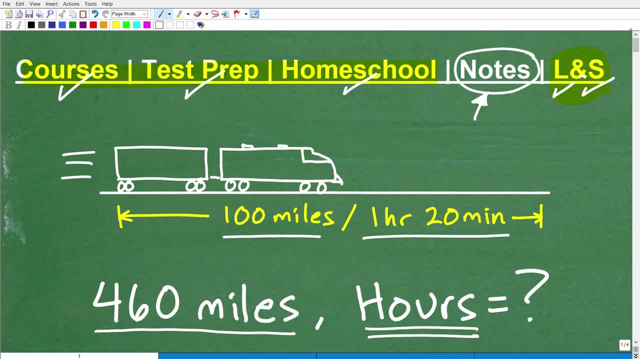 So if you need additional help with these basic kind of algebra word problems, I'm going to go ahead and point you towards my algebra one course in my math help program. Of course I cover word problems in my pre-algebra course as well.